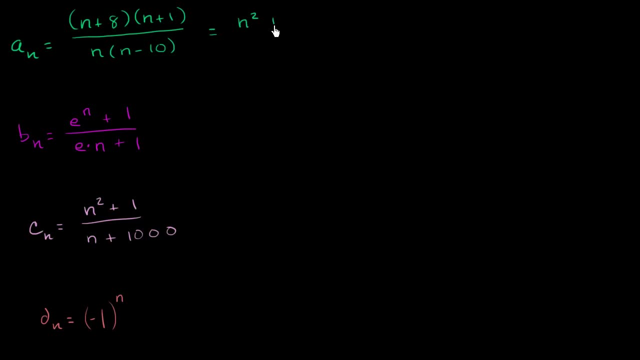 n times 1 is 1n plus 8n is 9n, So 9n, And then 8 times 1 is 8.. So the numerator is n squared plus 9n plus 8.. Denominator is n squared minus 10n. 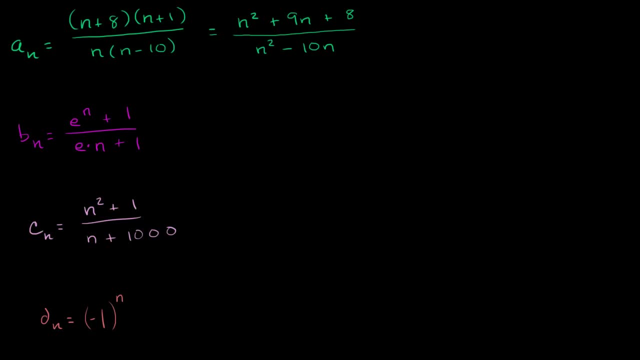 And one way to think about it is: n gets really, really, really, really, really large. What dominates in the numerator? this term is going to represent most of the value, and this term is going to represent most of the value as well. 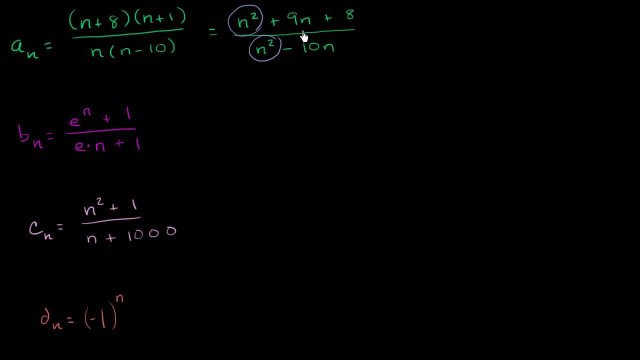 These other terms aren't going to grow. Obviously this 8 doesn't grow at all. But the n terms aren't going to go anywhere near as fast as the n squared terms, especially for large n's. So for very, very large n's, this: 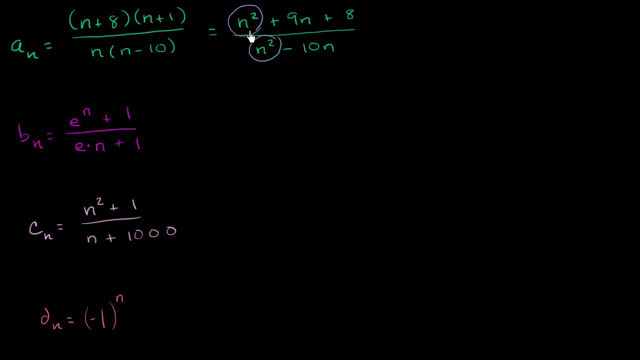 is really going to be approaching n squared over n squared, or 1.. So it's reasonable to say that this converges. So this one converges. And once again, I'm not vigorously proving it here, Actually I should say I'm not rigorously proving it over here. 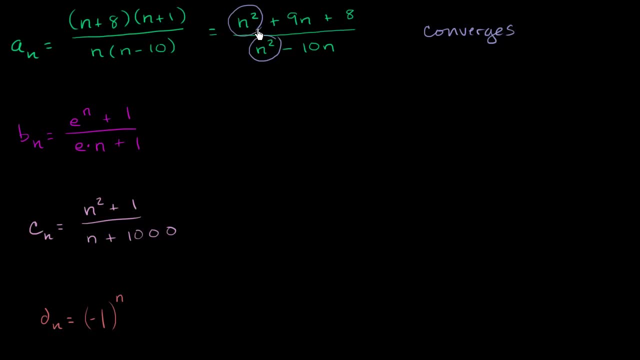 But the giveaway is that we have the same degree in the numerator and the denominator. So now let's look at this one right over here. So here in the numerator I have e to the n power, And here I have e times n. 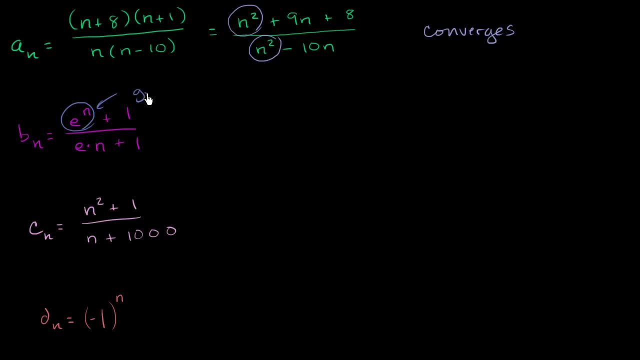 So this grows much faster. I mean, this is e to the n power. Imagine if, when you have this as 100. e to the 100th power is a ginormous number, e times 100 is well, that's just 100e. 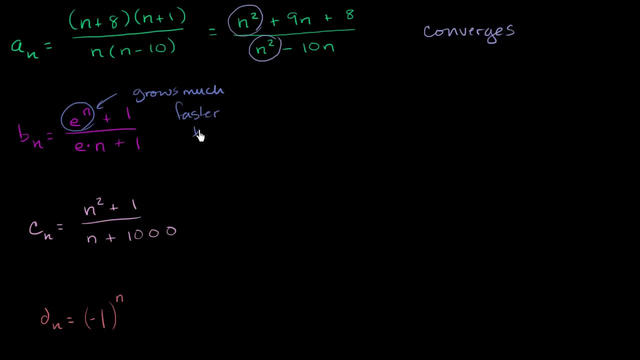 It grows much faster than this right over here. So this thing is just going to balloon, This is going to go to infinity. So we could say this diverges. Now let's look at this one right over here. Well, we have a higher degree in the numerator. 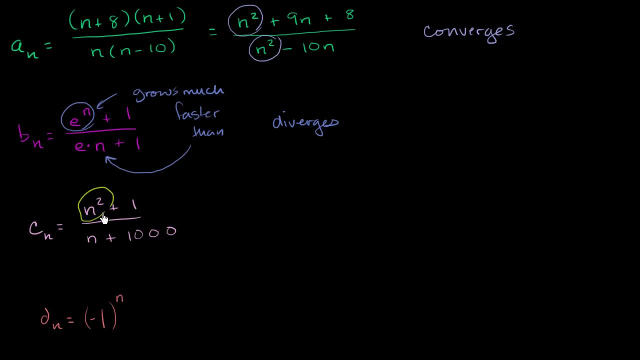 than we have in the denominator. n squared obviously, is going to grow much faster than n. So, for the same reason as the b sub n sequence, this thing is going to diverge: The numerator is going to grow much faster than the denominator. 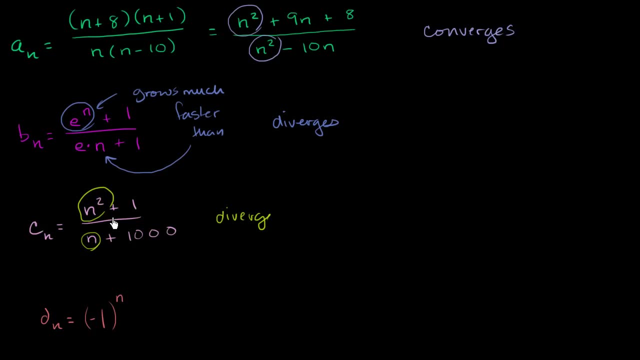 Or another way to think about it. the limit as n approaches infinity is going to be infinity. This thing is going to go to infinity. Now let's think about this right over here. So as we increase n, so we could even think about what.